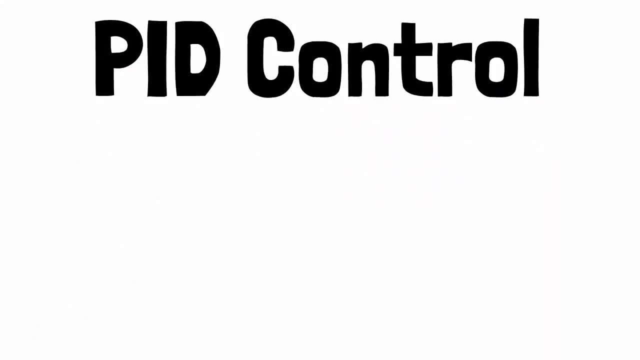 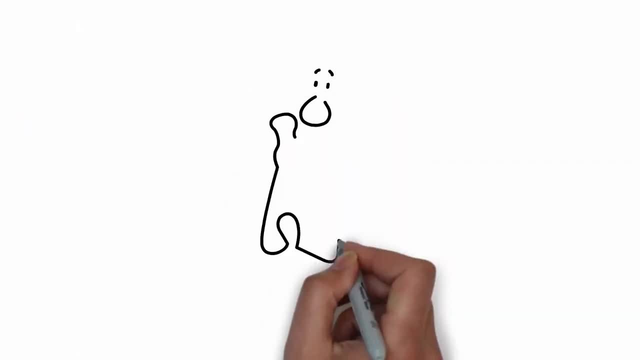 PID control in its simplest form is a method used in control systems to maintain a process variable at a desired set point by manipulating an output. Let's get into exactly how this works, and later in the video I'll show you some software that will help you visualize what you have learned. 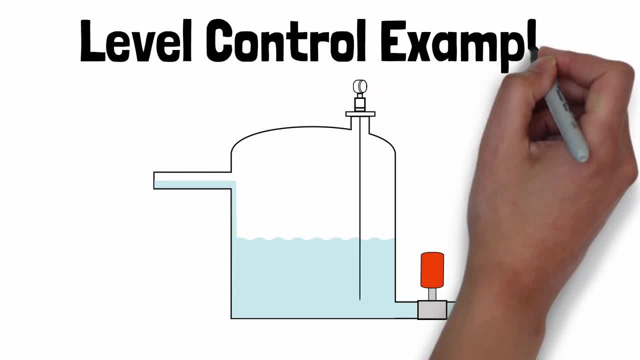 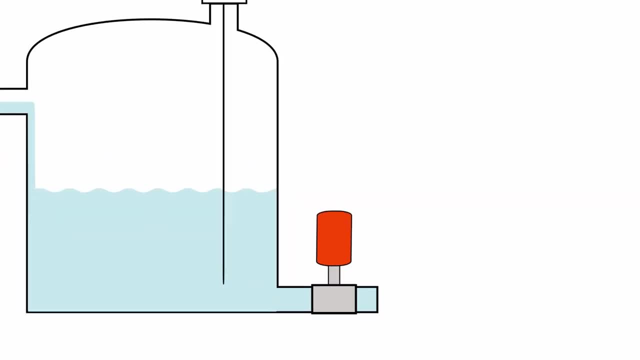 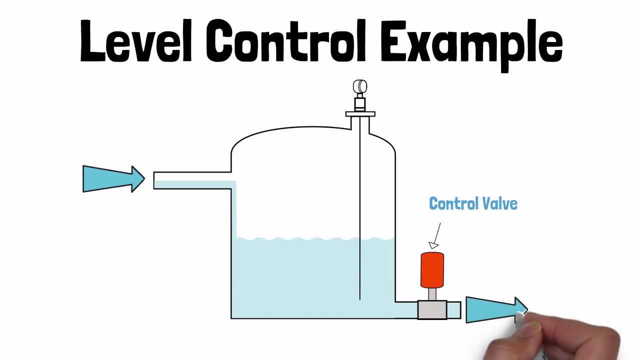 Let's look at a level control example and how PID control might be used. We have a vessel that has a continuous flow of liquid coming into the vessel from the process. On the outlet pipework of the vessel we have a control valve that will vary the flow of liquid traveling through the 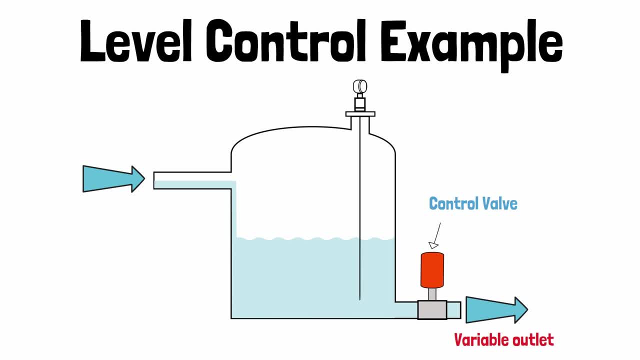 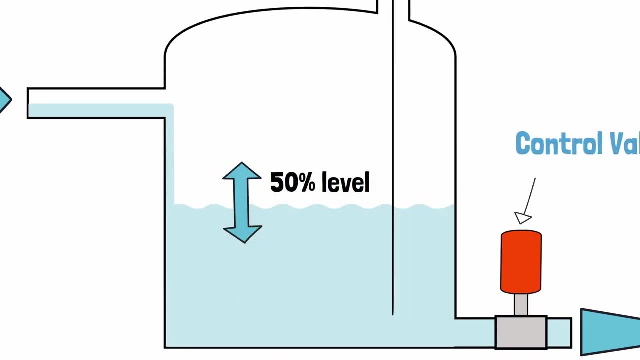 valve and out of the vessel, depending on the valve's position. This in turn will adjust the level in the vessel, assuming the inlet flow from the process is steady and not changing. Say, we want to control the level of liquid in the vessel at 50 percent. How would a PID control 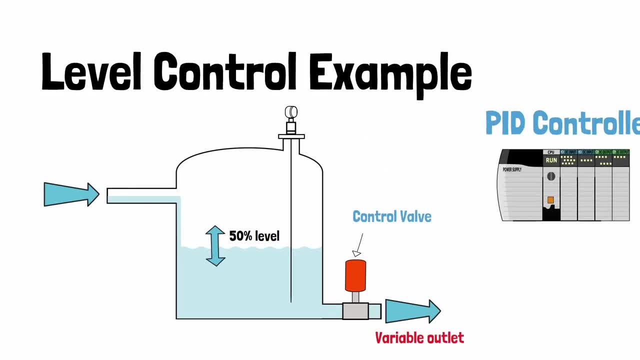 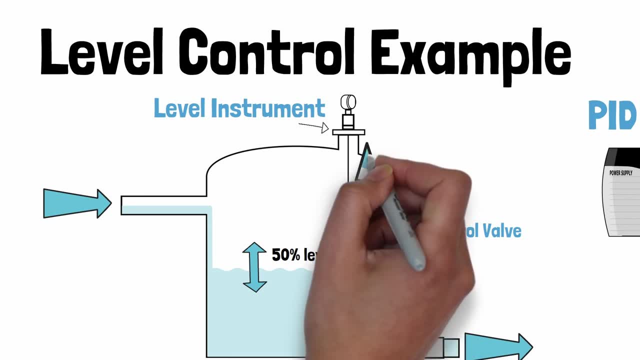 be used to control the level in this vessel. Well, first we need a level instrument that is used to continuously monitor the level of the liquid in the vessel. Let's say this is a radar instrument that gives a 4 to 20 milliamp signal. that represents 0 to 100 percent level of the 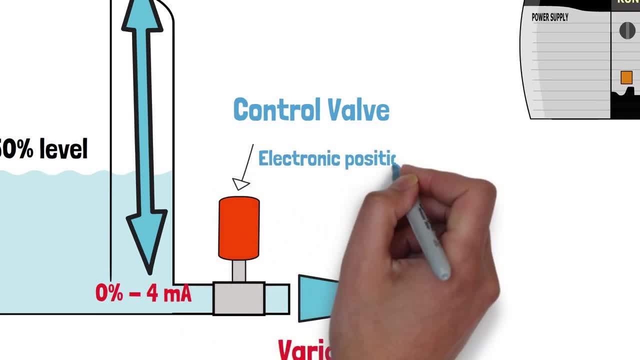 vessel. We then have an electronic positioner on our outlet control valve that takes a 4 to 20 milliamp signal- 4 milliamps for fully closed and 20 milliamps for fully open. Both our level instrument and control valve would be connected to a PID controller. 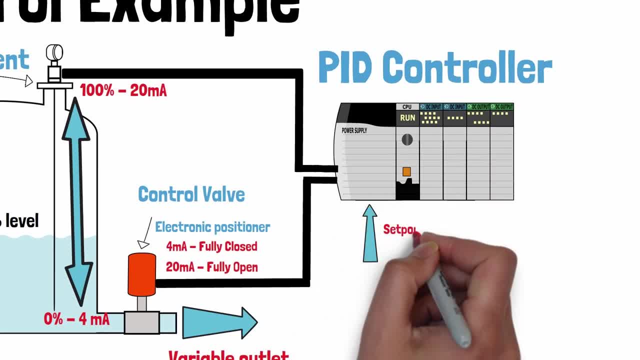 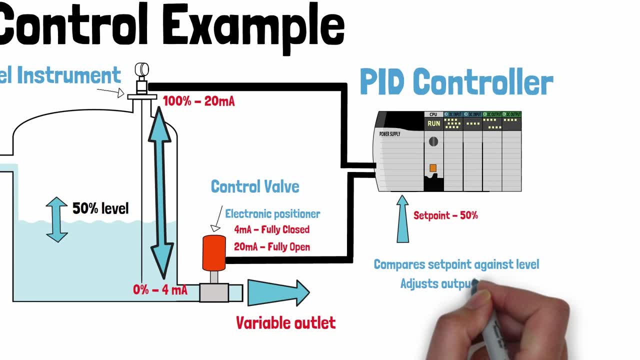 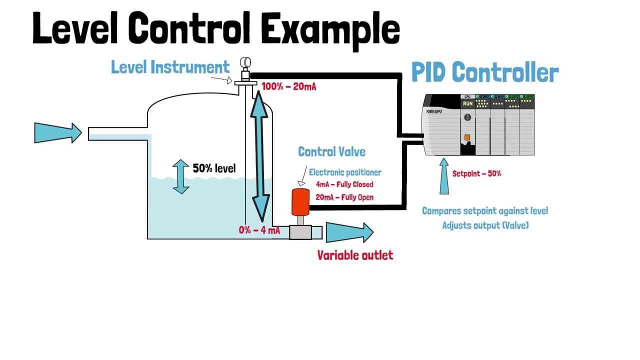 We then provide the controller with our set point: 50 percent. The controller then compares the set point to the process variable and, depending on the difference or the error, will adjust the output demand on the control valve. This in turn will move the valve and start to adjust the level in. 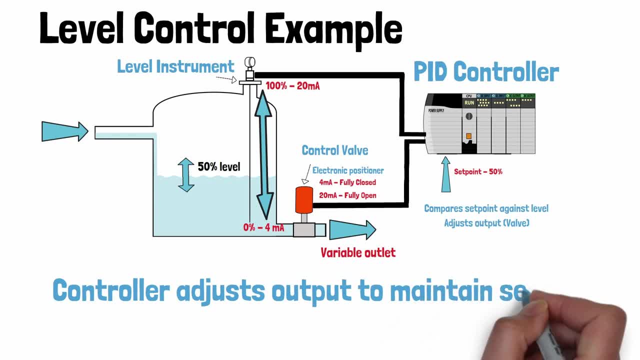 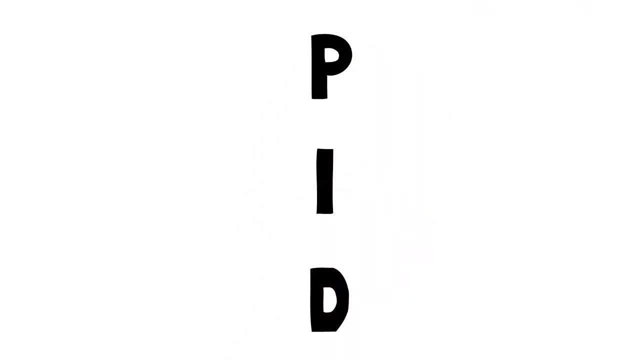 the vessel. This change is detected by the transmitter. The controller works to minimize the error and tries to control the process condition as close to the set point as possible. This is what we call closed loop control. PID controllers are called PID due to three 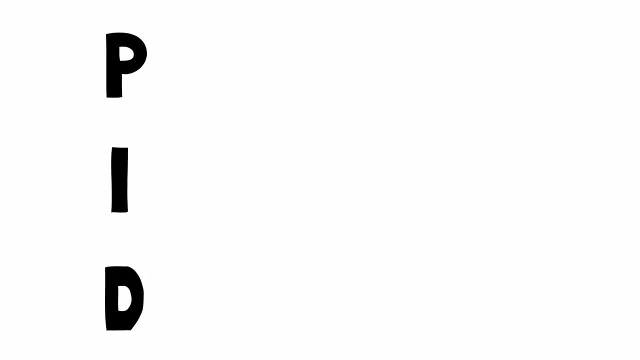 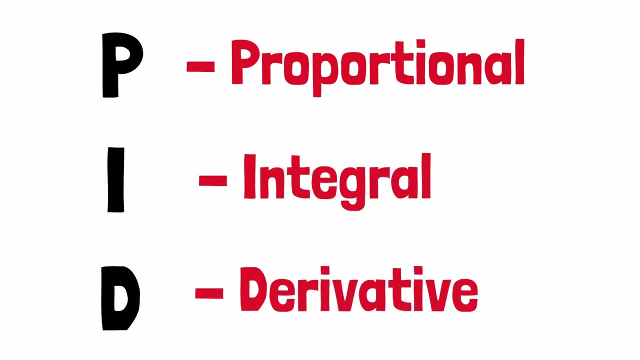 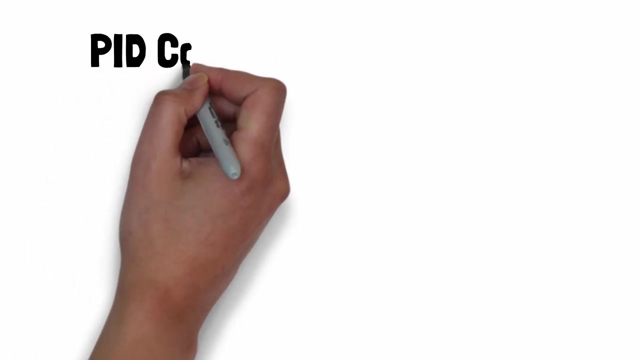 different values that are used to adjust the behavior of the controller. This is proportional, integral and derivative functions. These values, or multipliers, all change the way the controller changes the output in relation to the error. To understand what the individual functions are doing, we need to have clear in our mind. 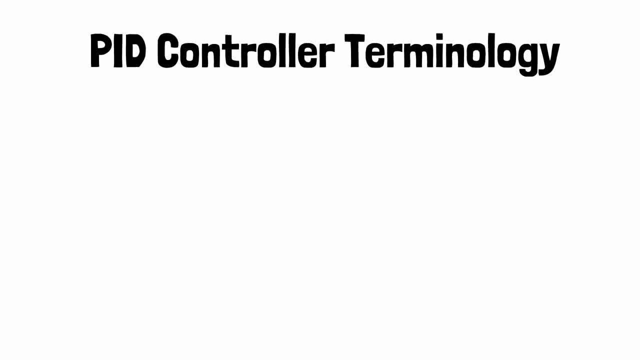 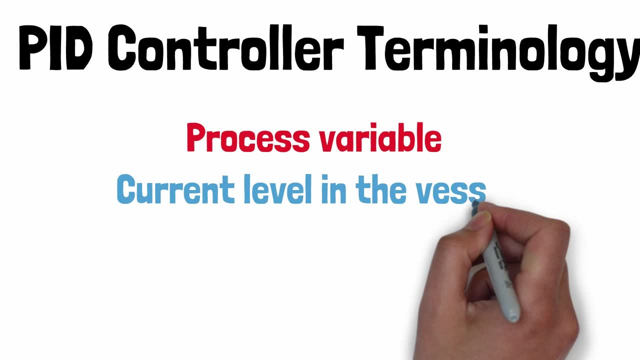 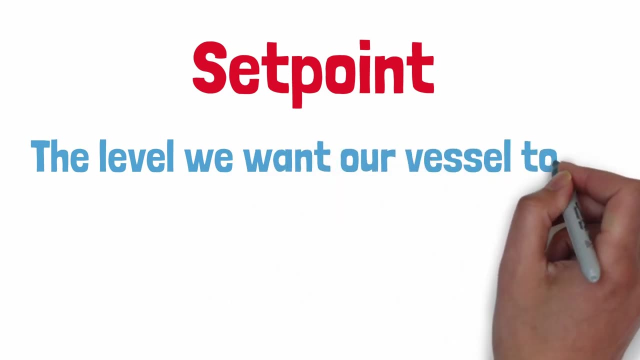 the terms that are manipulated or used by the controller. Process variable: The current level of the vessel in percentage, as detected by our transmitter. Set point: The value we want to control our vessel at in percentage. This would be manually entered into the controller by a plant. 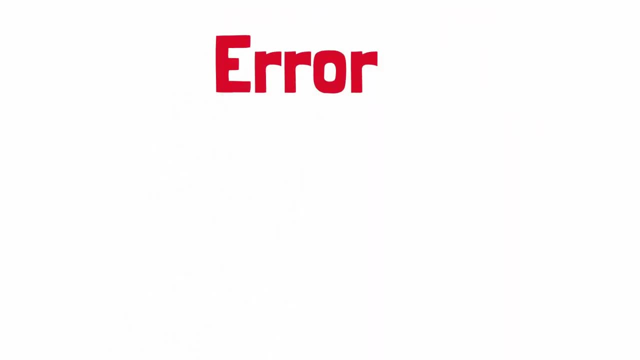 operator Error. This is the difference between the value of the controller and the value of the set point and current process variable. Say, we have a set point of 50% but our level is currently reading 60%. This will be a 10% error Output. The result of the PID controller calculation. 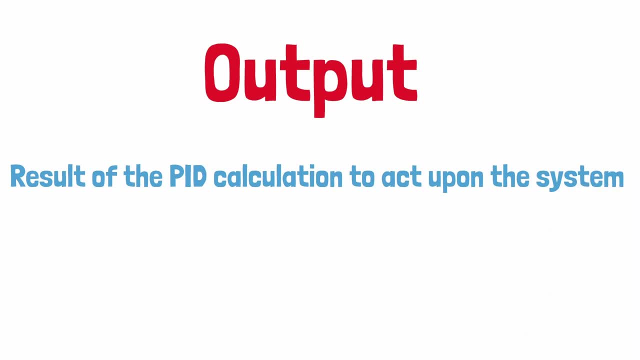 In our example this will be between 4 and 20 milliamps. that is connected to our control valve. As the output changes, so does the valve and thus changes the level in the vessel. Now we understand the inputs and outputs of our controller. 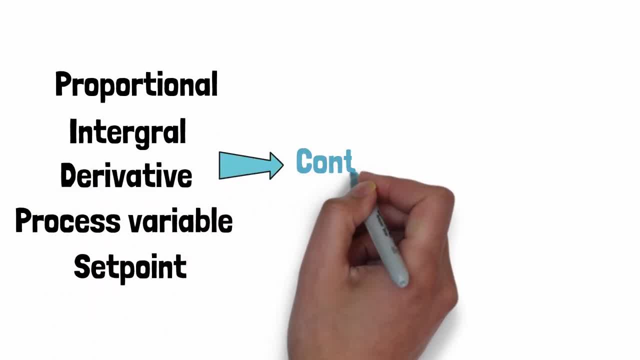 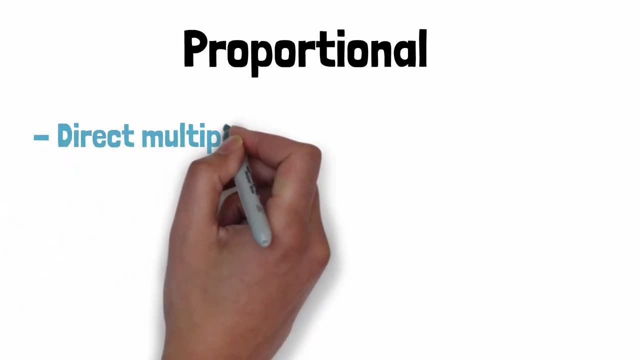 let's look at the PID terms and how they all interact. The three multipliers, or gains of PID control, are used in combination to change the output of the controller. in relation to the error Proportional term, The proportional value works as a direct 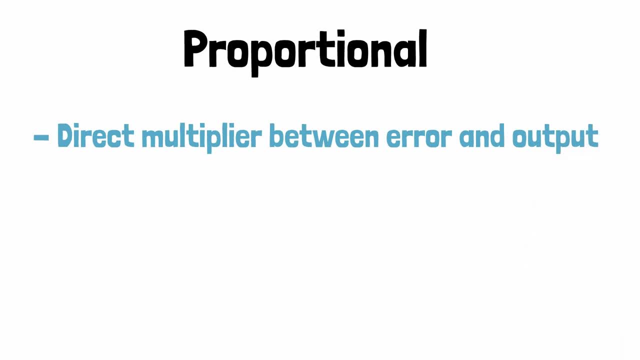 multiplier between error and output. The controller will change the output proportional to the error between set point and measured value. A low proportional value will mean only small changes to the output are made in response to the error. This would lead to a slow acting or less sensitive controller. Large proportional gains will cause small errors to enact large. 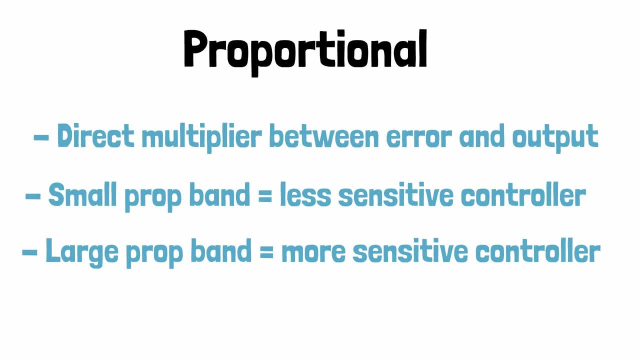 changes to the output and make the controller more sensitive. Proportional control can be used on its own without the use of integral or derivative bands. However, because an error is required to change the output with proportional control, this will lead to a steady state error where the process variable will not exactly meet. 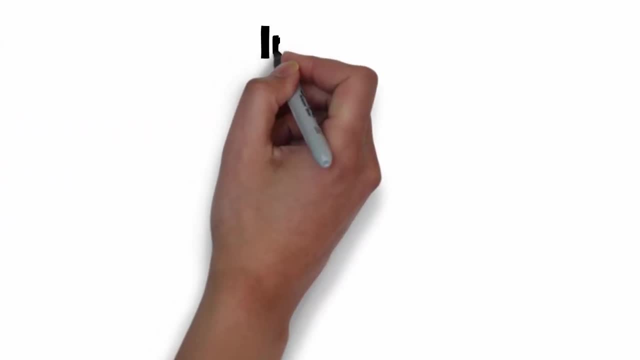 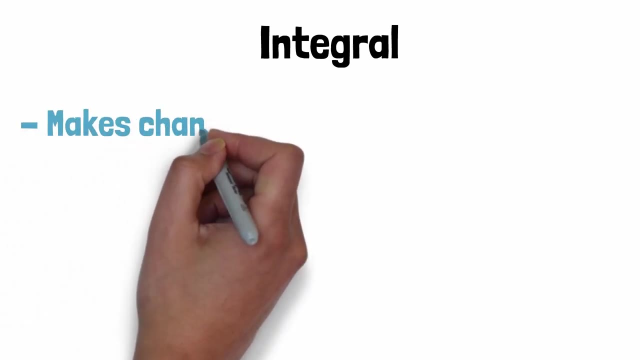 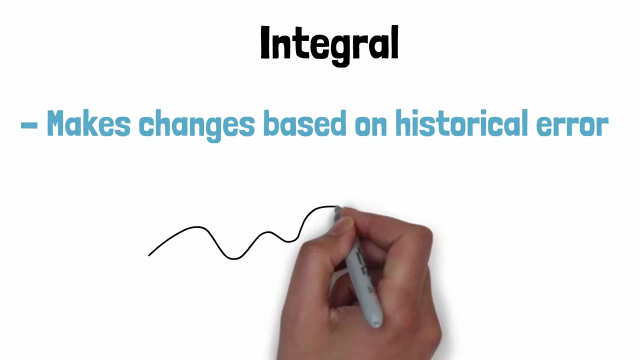 the set point. This is where the other terms are required. Integral Term, where proportional band makes changes based on the current error. integral band makes changes based on the error over time. If you're familiar with calculus, this might make sense, as integration is used to find the area under a function when plotted. 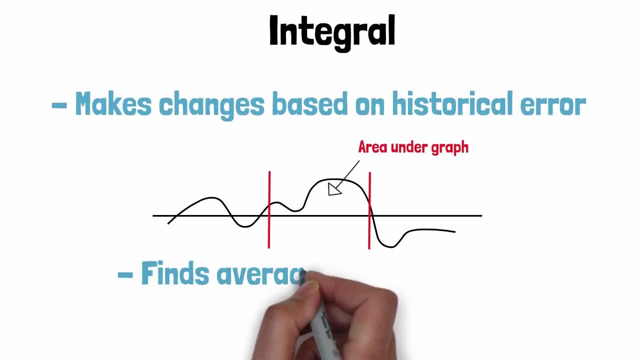 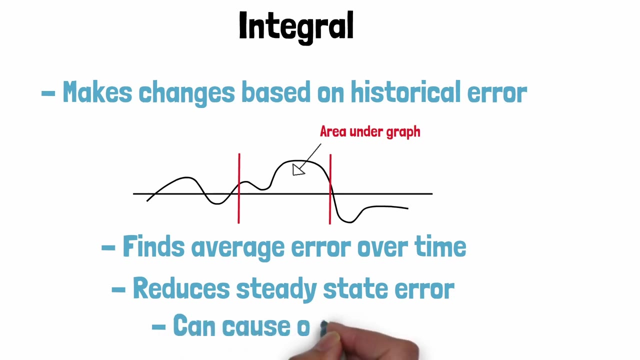 on a graph. In the same way, the integral band is used to find the average error over a set time period. This will reduce the steady state error caused by the proportional band over time. One of the issues with integral band is because integral band makes changes to the output. 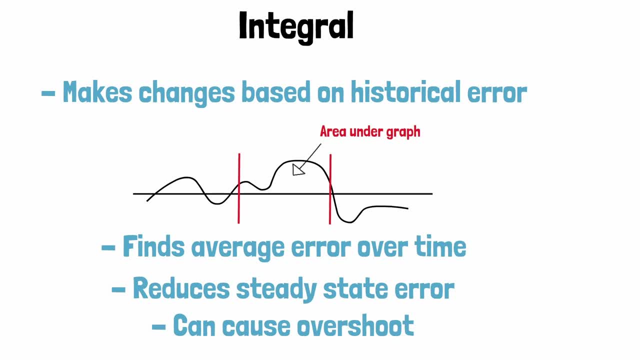 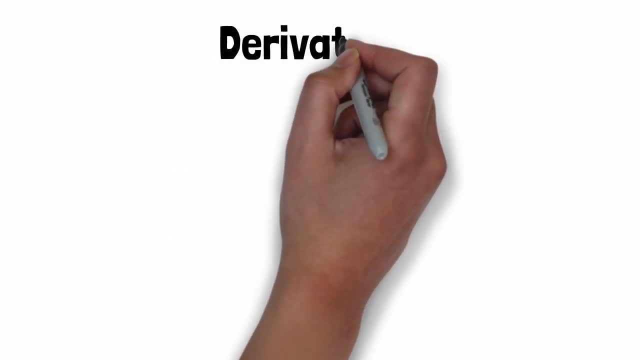 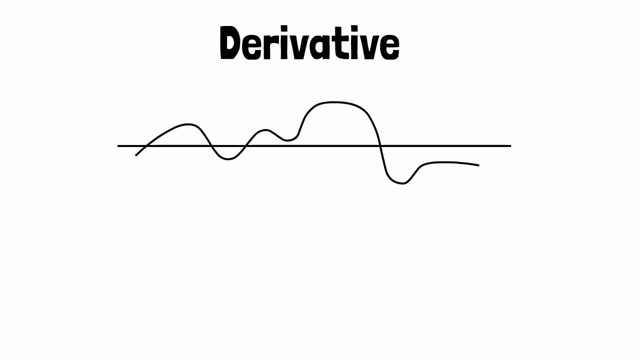 based on historical error Overshoot. compensation can occur where changes are being made to an error that doesn't currently exist. Derivative- Again, a little understanding of calculus helps us to understand the derivative term. If we differentiate a mathematical function, we end up with a formula. 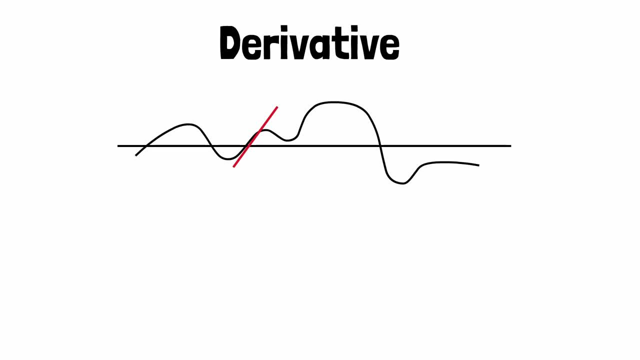 that can be used to calculate the gradient of that function. Or, simply put, we can use differentiation to predict if a graph is moving up, down or is flat. In the same way, the derivative function is used to indicate the rate of change of the error over time. 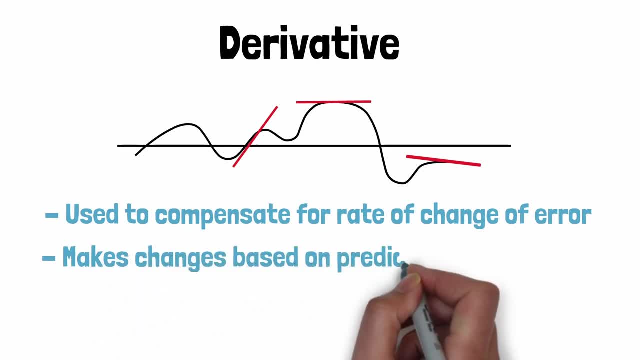 Where integral is based on the past error, derivative is used to predict the future state of the error based on how quickly or slowly the error is changing, and make changes to the output to reduce the error. This can help prevent overshoot. Derivative isn't often used but can. 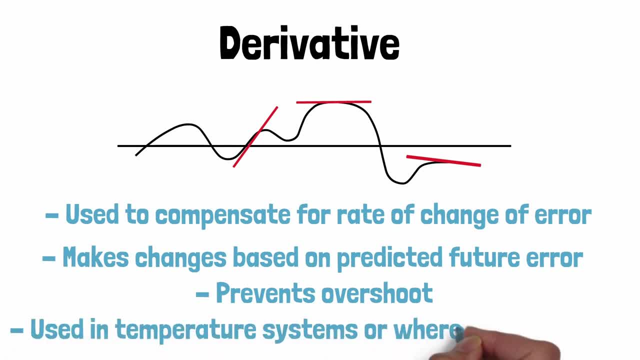 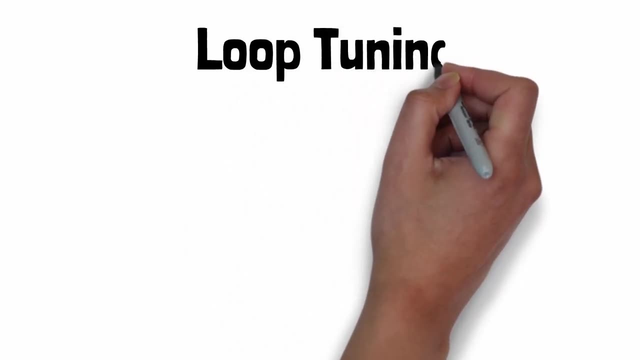 be found in examples such as temperature control. This is because temperature control loops have a dramatic lag between an output change and its effect on the process variable. So how do we decide what to set these values at? Setting the PID values is done via a process. 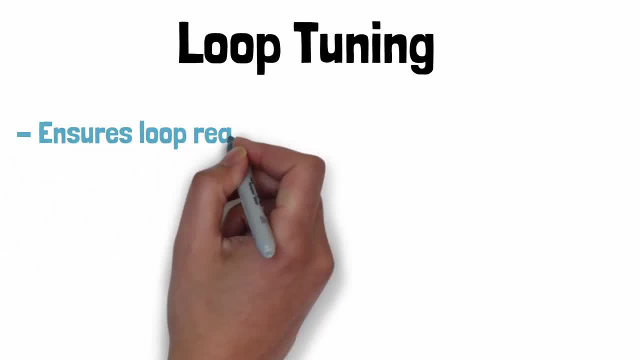 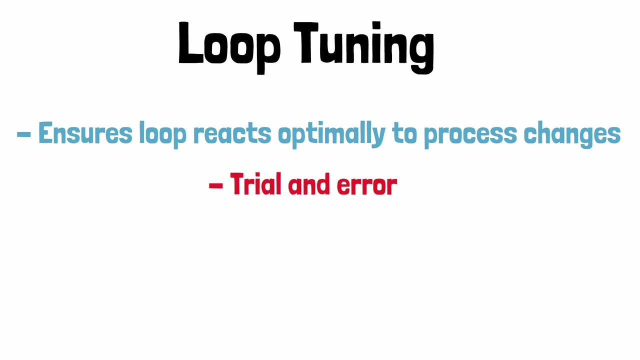 called loop tuning. The aim of tuning is to ensure the controller reacts to changes in process conditions and the error is minimized in the most efficient manner. There are multiple methods that can be used to tune a PID loop. One of the common ways this is done is with a trial and error. 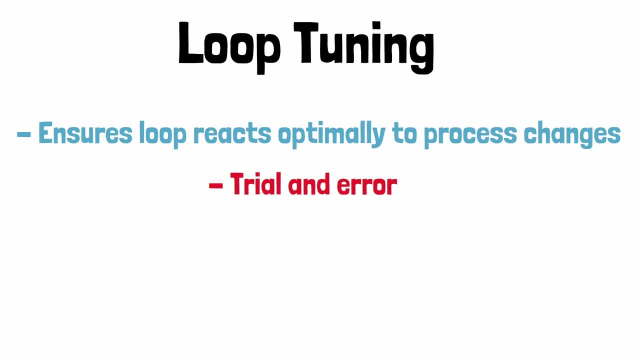 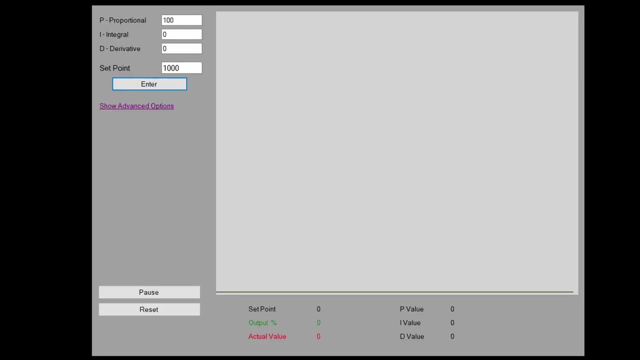 approach by someone with a lot of experience in loop tuning. There are more theoretical and math-driven approaches, such as the Zeiger-Nichols tuning method. Auto-tuning software can be used that will dynamically make system changes to decide the PID settings. This is useful where a business might not have easy access to people with experience in loop tuning. 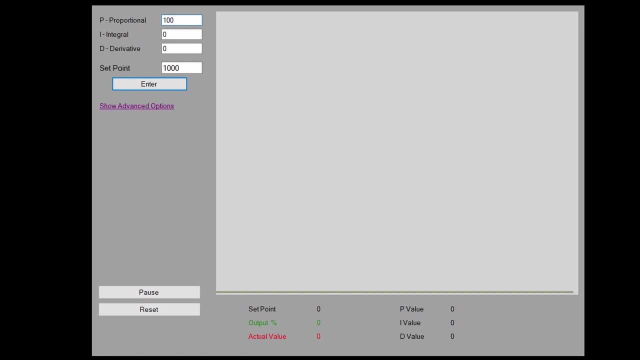 Let's look at some simulation software for PID control that will hopefully make this more clear. This software I found on the Microsoft Store. This software lets us try different PID settings and simulate its effect on a control loop. Don't worry too much about the numbers we're going to use. 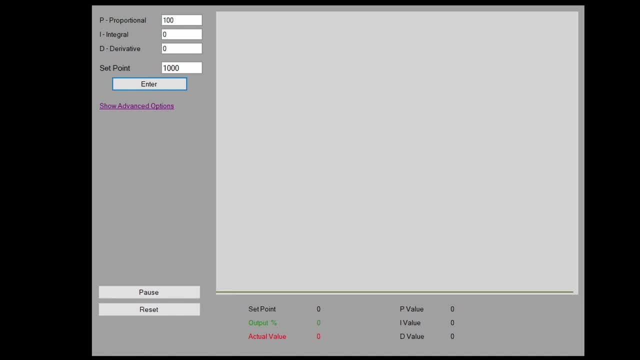 We're just going to use them to get an understanding of the effect of changing the PID settings Up. here is where we input our PID settings, so our proportional, integral and derivative, And here we can put the setpoint in. So, as I said, don't worry too much about the numbers, but we've put a setpoint of 1000 in and a proportional value of 100. 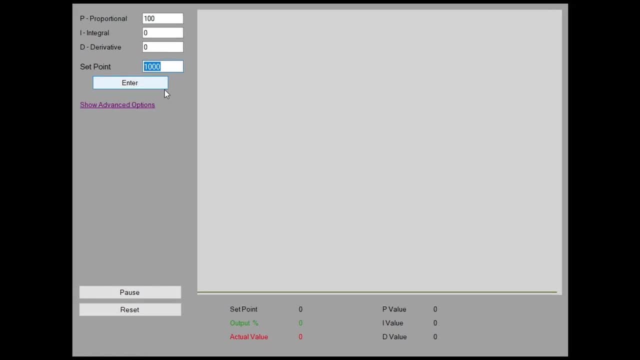 If we start this going, the control loop will try to control to the setpoint And we get 3 lines which are a visual representation of the control loop. So we have our black line, which is the setpoint. As you can see here it's 1000.. 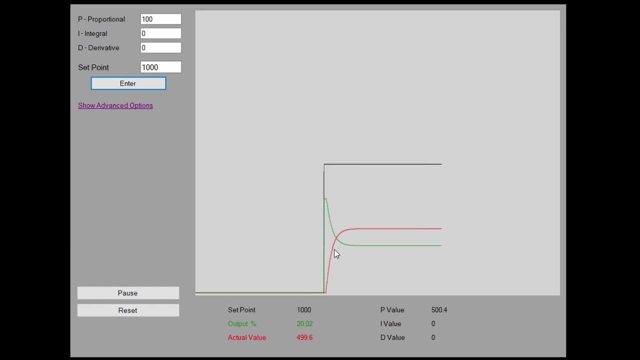 We have our red line, which is our actual value. This is the same as our PV- and then our level. example would be the level the vessel at this current time. The green line is the output of the PID loop. So, depending on the error, the PID loop will make some control adjustments and this is our output. So, again, if 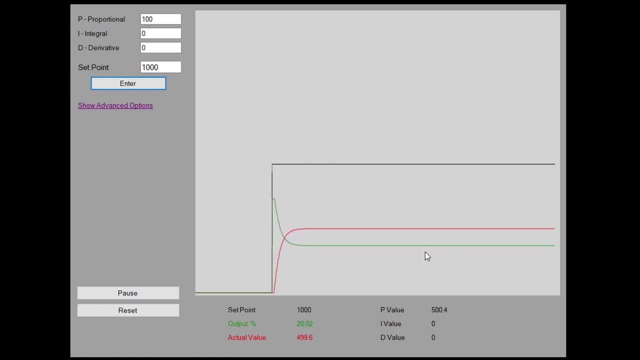 we're thinking of our level example, level control example. this would be the output to the control valve. So here you can see we have a set point of a thousand and just a proportional band of one thousand. If we start this graph in we can see here the proportional band is set quite high at. 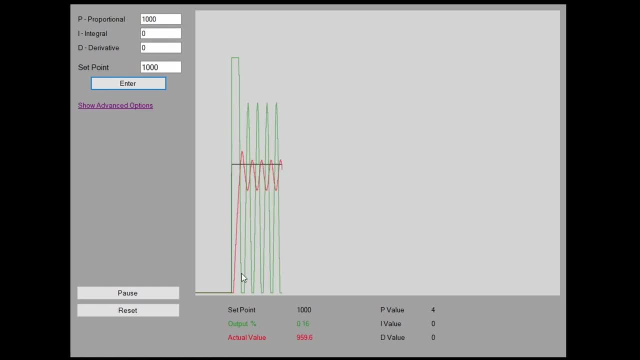 a thousand and this is causing the output to swing between nought and a hundred percent. So in our real-life example, our valve would be going from fully open to fully closed, and the effect that this is actually having on the level, which is our actual value here you can see it's kind of. 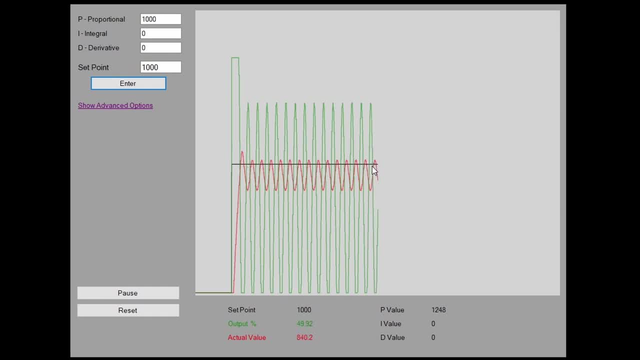 swinging above and below the set point, which is the black line. So this isn't good control. this is what we want is a nice smooth line. but we're not getting that here. we're just getting this, this constant swinging up and down, because our proportional band is too high. So let's make an adjustment here. so if we put our prop band to 500, press. 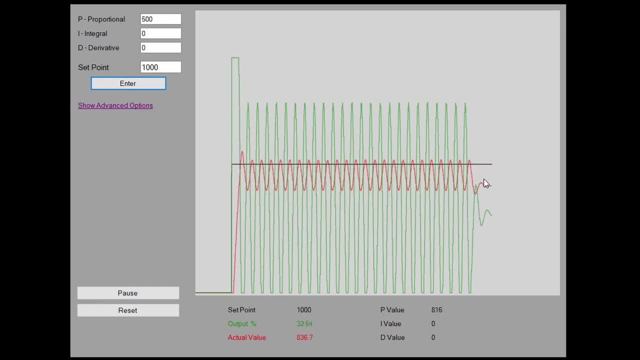 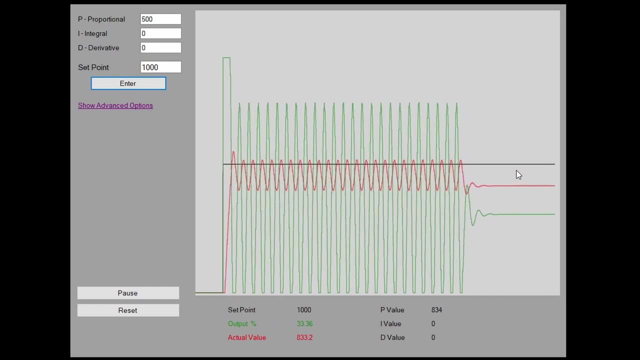 enter and give this time. So you can see our output has stopped swinging from a nought to a hundred percent and has somewhat settled out, And what this has led to is a steady state error. So you can see on our graph: we've got our set point. 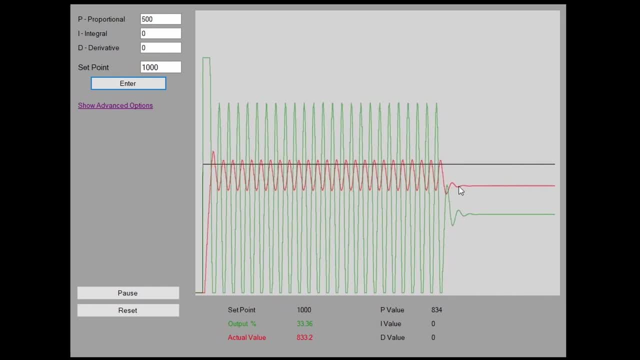 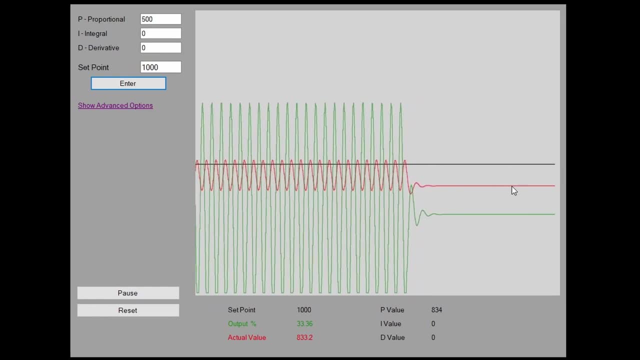 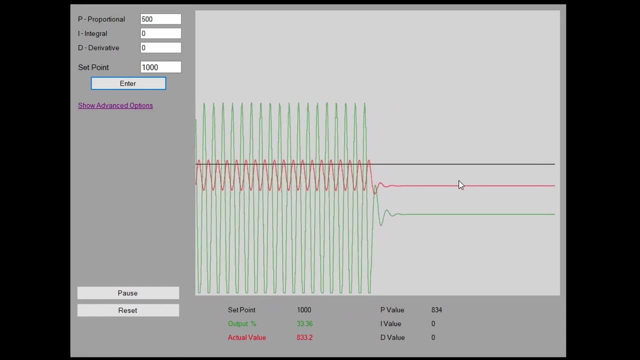 which is 1000, and our actual value has settled out at 833.. So we've got we've got an offset of around 170, and this is because we're just using proportional band. So with proportional band we'll always end up with this error, as we spoke about before, because the output is being adjusted. 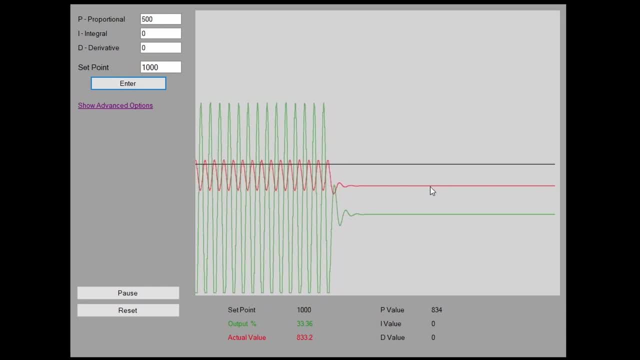 in proportion to that. So we've got a steady state error and we've got a steady state error. so once we've got this fixed error and it's settled down, there's no way of getting rid of this without using integral band. Okay, so we've just let this settle out so we can see our output. 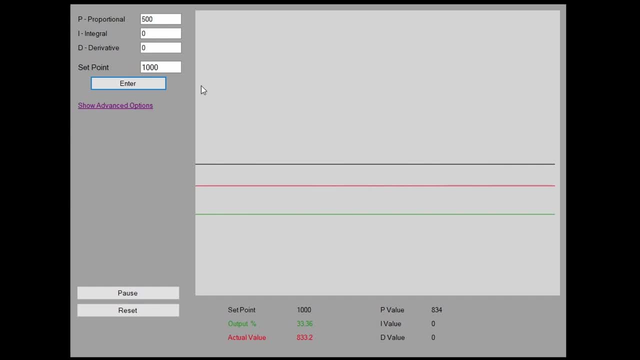 position, actual value and our set point. So if we had a little bit of integral band, not much here. we're just going to go 10 and we'll press enter. So now you'll notice that the output is starting to change and this is because we've got this cumulative error over time. So we've got this. 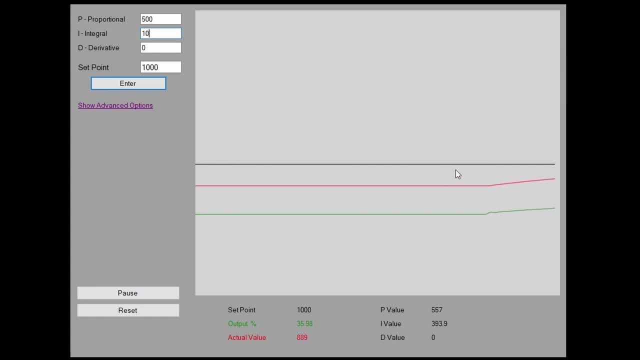 error that we've- the steady state error that we've spoke about- and it's slowly being closed because of the effect of the cumulative error. So if we look at our i value- this bottom right hand side down here, you see that this value is increasing and that's due to the cumulative error. 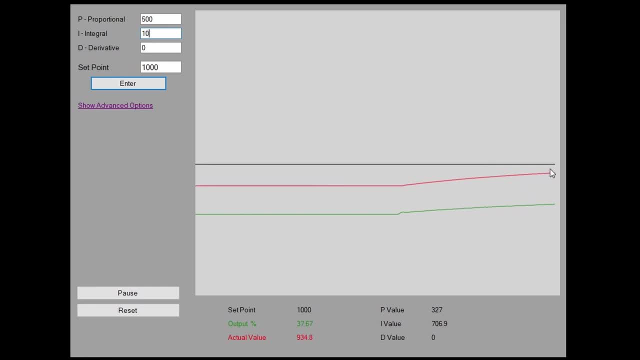 That's still going up and it's very slow, but we're heading towards our set point. Our red line is approaching the black line. If we just change this and just increase the speed a bit- let's say not 50, let's go 100.. We press enter here- you can see it's making a bigger change. 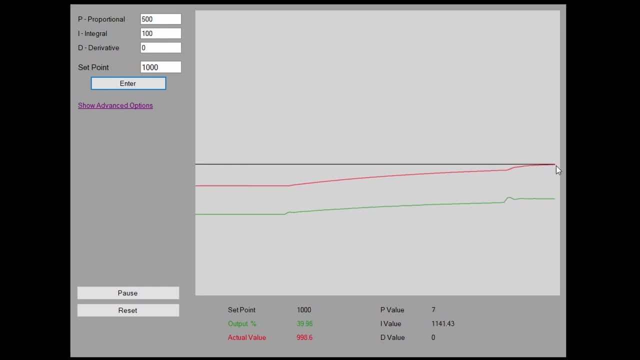 our i value is still increasing and our actual value is rapidly approaching the set point. So here we're settling out 999.8 and there we go, we've hit the actual value of a thousand. so we're controlling dead on there. Okay, so to talk about the derivative functions. So it's harder to demonstrate the effect of. 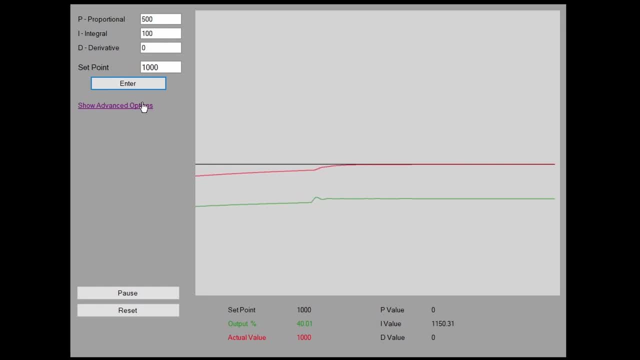 derivative using this software. but we can use the advanced options here in this software and to add a change in the process variable and see the response without the derivative band, and then we'll put some derivative band on and we'll see the effect with it. So if we simulate a load here just decreasing by 500.. 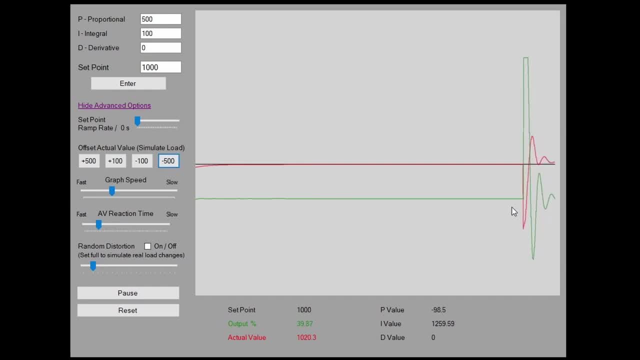 So let's just put a load. basically we've moved our output and then our control loop is trying to control that. So you see, we have this overshoot action where the actual valve shoots above the set point and then bounces and then settles out. 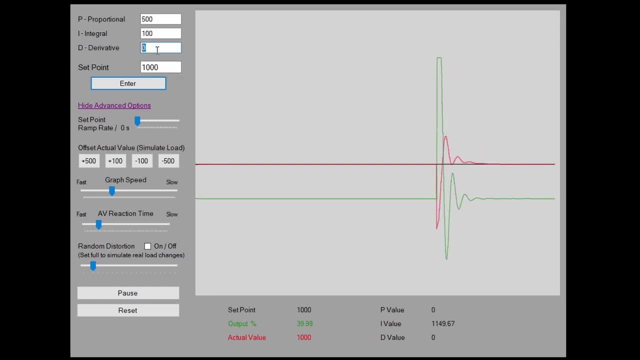 If we add some derivative function and then we put the same load on the system. so again this minus 500, so you can see, here we have the same overshoot, but instead of getting this big bounce effect it's actually tapered off the control, and it's nice and controlled as it comes back to that set point. 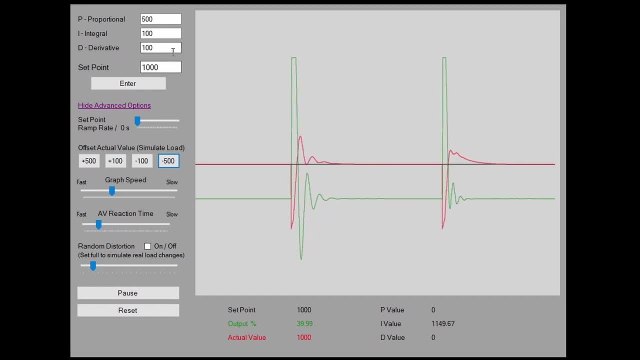 So that's the effect of derivative. it basically helps prevent, overshoot, again by looking at the rate of change of the error. Okay, so hopefully that's given you a little bit of a visual understanding of what we've learnt. If you want to use this software yourself, I'll put a link down in the description for the Microsoft store. 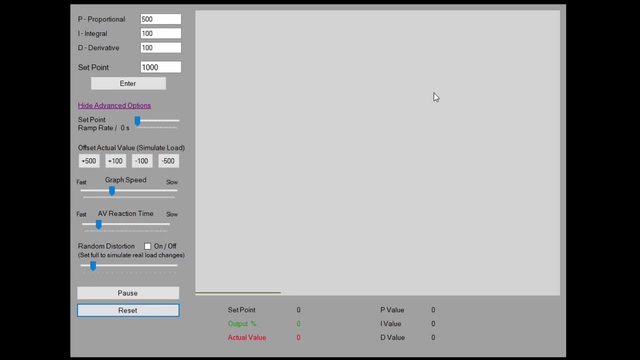 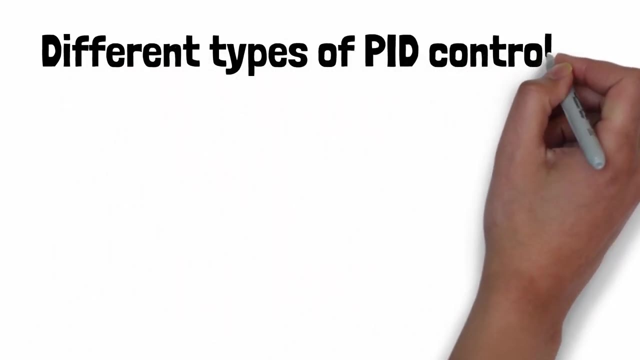 Just a note. I have a Xero affiliation with the creator of this software. I just found it and thought it would be useful to teach you all and show you a real life example of PID control without being out on a process plant. Just thought I would add here at the end: in industry you might come across PID controllers in numerous formats. 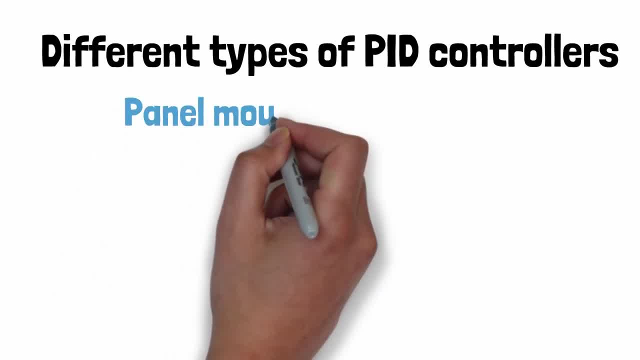 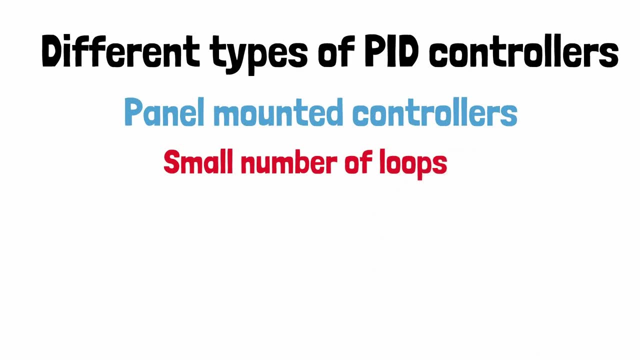 The common types I've come across is a standalone controller. They're usually panel mounted. they're used usually to control maybe one or two loops. The more common format in larger industries and applications is for the PID controller to exist in the software of a PLC that has inputs and outputs that are connected to the field equipment.